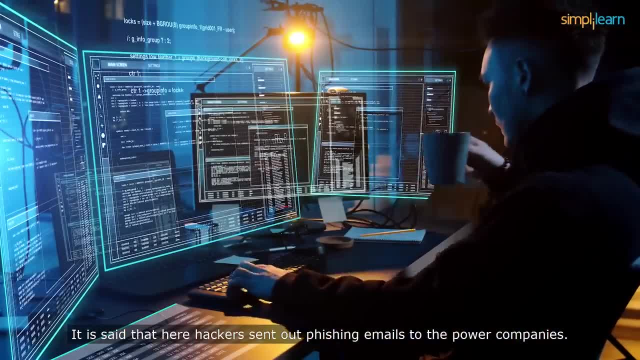 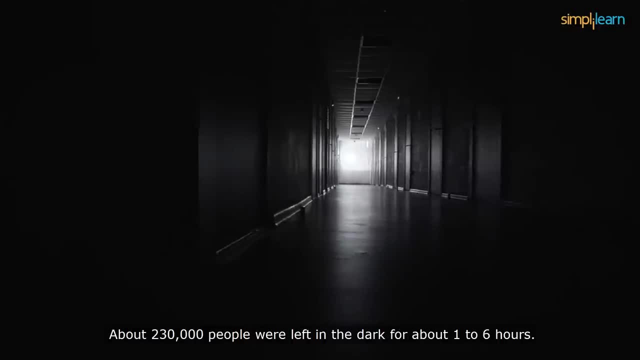 It is said that here, hackers sent out phishing emails to the power companies. 30 substations were switched off and about 230,000 people were left in the dark for about 1 to 6 hours. US investigators believed that Russia-based hackers were responsible for this. 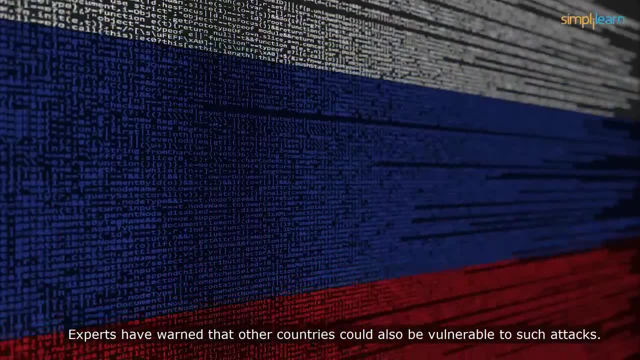 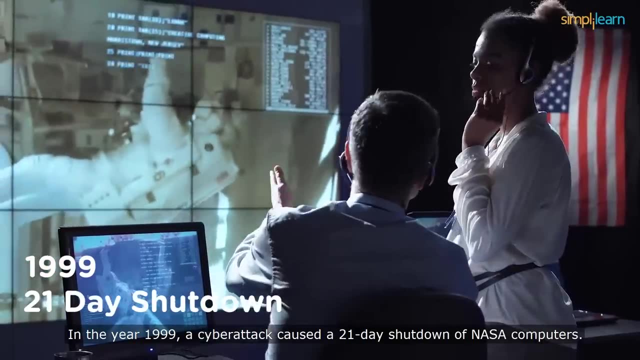 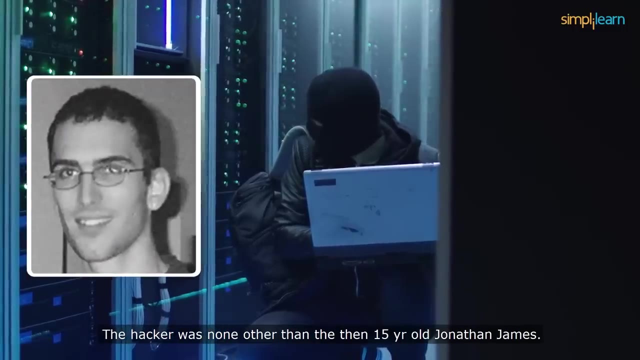 Experts have warned that other countries could also be vulnerable to such attacks. Let's see what we have at number 8.. In the year 1999, a cyberattack caused a 21-day shock. The hacker was none other than the then 15-year-old Jonathan James. 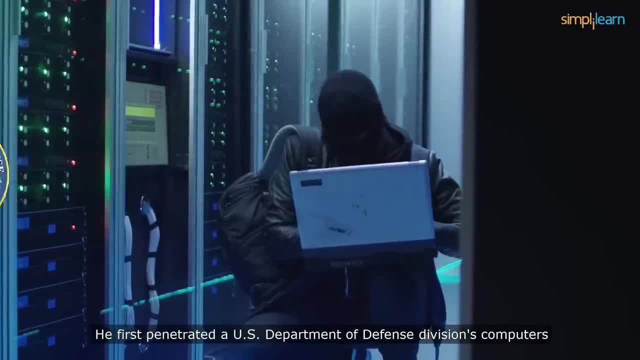 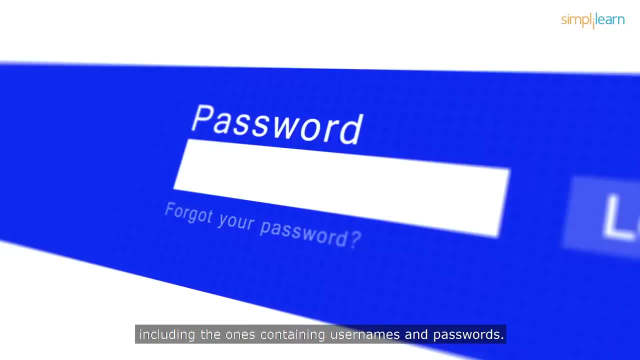 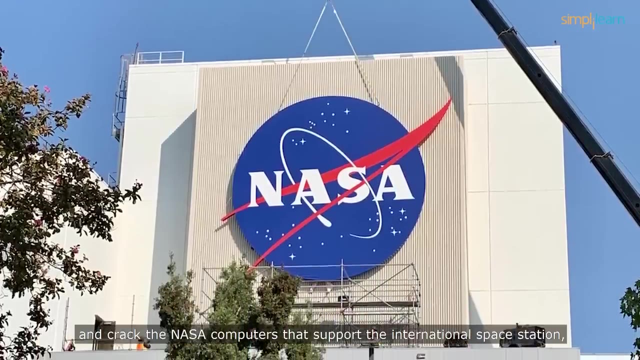 He first penetrated US Department of Defense Division's computers and installed a backdoor on its servers. This allowed him to intercept more than a thousand government emails, including the ones containing usernames and passwords. This helped James steal a piece of NASA software and crack the NASA computers that support. 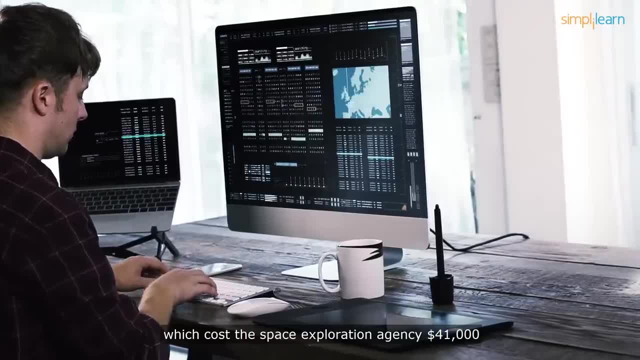 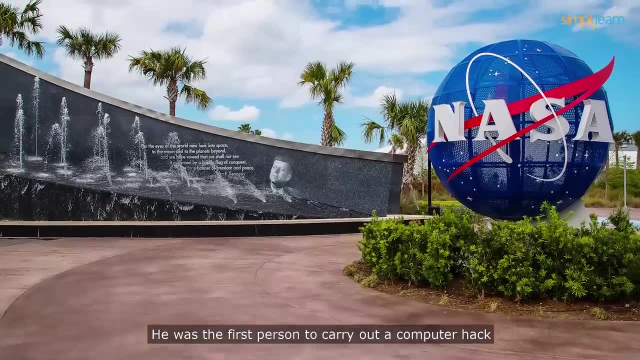 the International Space Station, which caused a space explosion. He also stole the space exploration agency's $41,000, as systems were shut down for three weeks. He was the first person to carry out a computer hack against the American Space Agency. Let's now move on to the next attack. 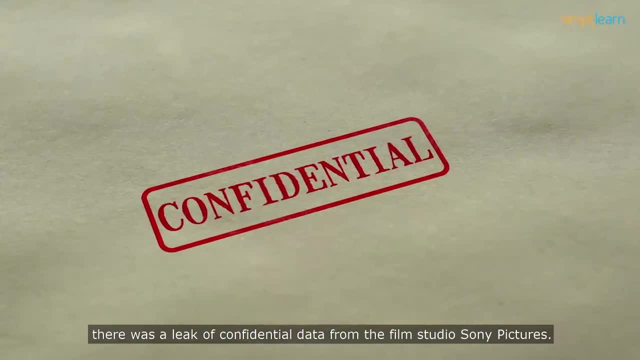 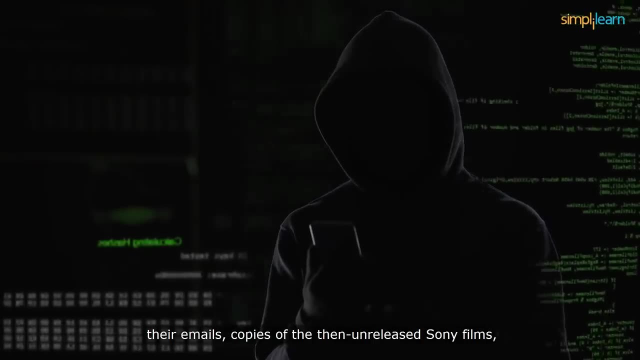 In late November 2014,. there was a leak of confidential data from the film studio of Sony Pictures. Information about Sony Pictures' employees, their emails, copies of the then-unreleased Sony films, future propositions and other crucial data were leaked. 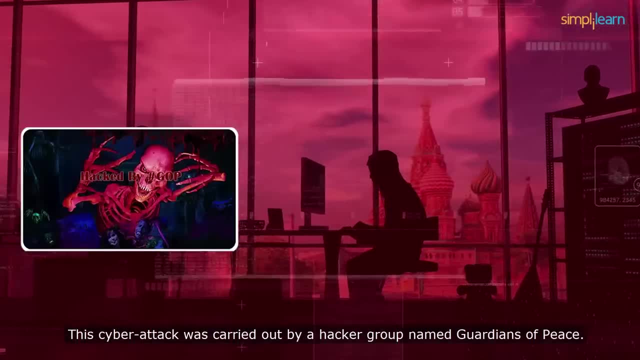 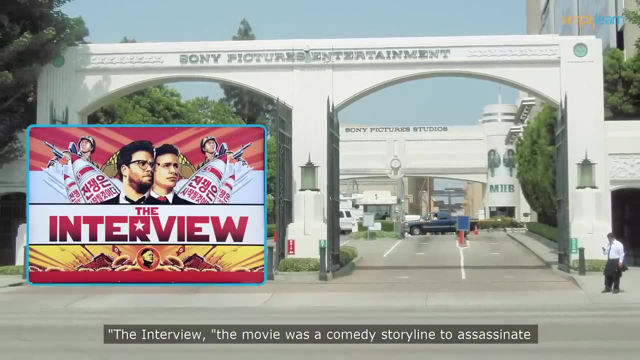 This cyberattack was carried out by a hacker group named Guardians of Peace. So what did the hackers want? Well, they demanded that Sony withdraw its then-upcoming movie, The Interview. This movie was a comedy story line to assassinate the North Korean leader, Kim Jong Un. 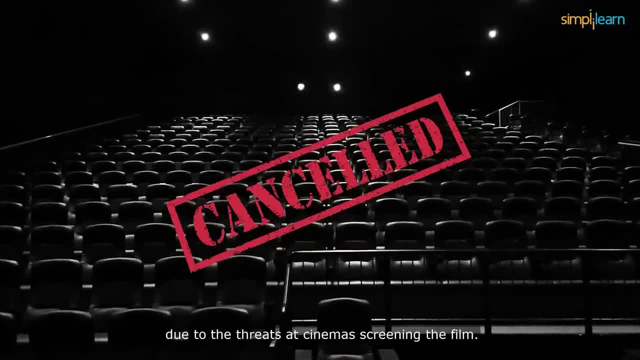 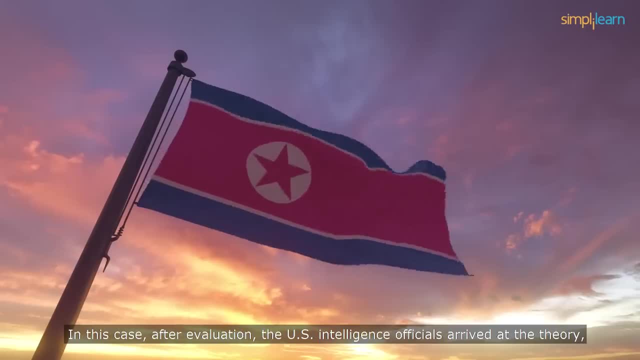 Sony then decided to cancel the film's theatrical release due to the threats at cinemas screening the movie. It is indeed hard to trace the roots of a cyberattack In this case. after evaluation, the US intelligence officials arrived at the theory that the attack 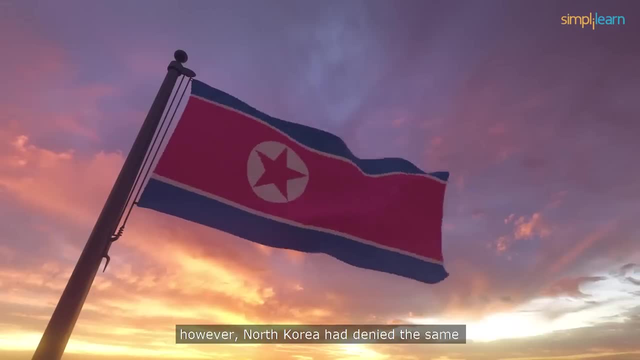 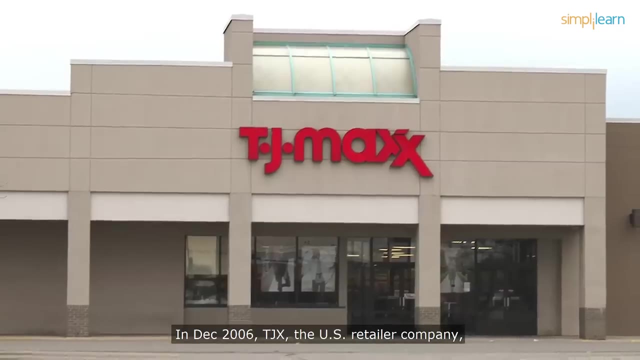 was, in a way, related to the movie, related to the government of North Korea. However, North Korea had denied the same. Moving on to our number 6.. In December 2006, TJX, the US retailer company, identified that 45.6 million debit and credit card details were stolen. 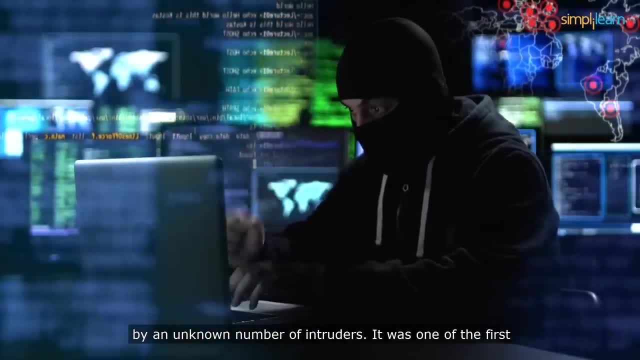 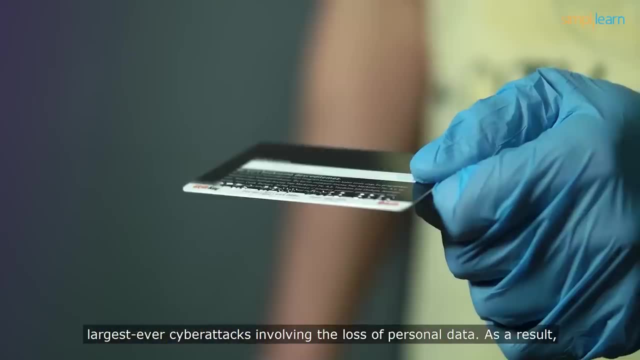 This happened from one of its systems over 18 months by an unknown number of intruders. It was one of the first largest ever cyberattacks involving the loss of personal data. As a result, banks in the affected regions had to re-issue and block thousands of payment cards. A group of hackers did this, Albert Gonzalez being the mastermind. The group was from Miami, the place where the TJX heist was believed to have originated. Reports said that the TJX data breach occurred because of weak web encryption at two of its Marshall stores in Miami. 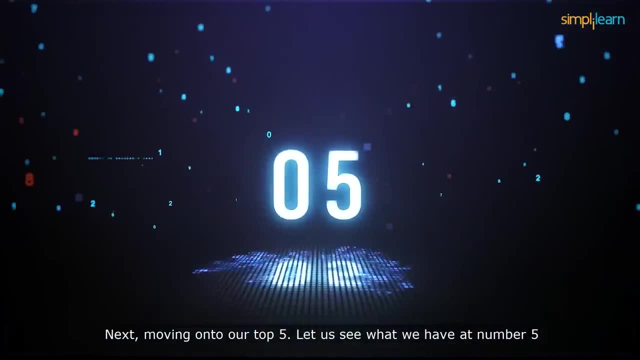 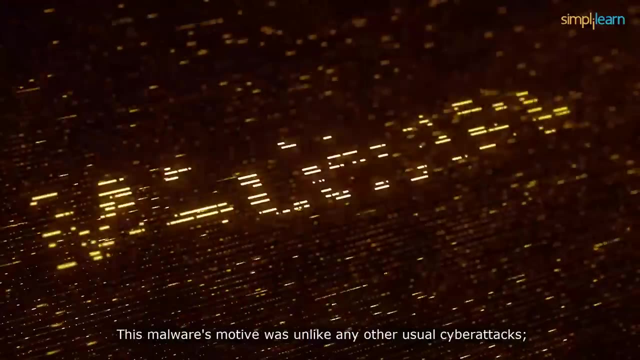 Next, moving on to our top 5, let us see what we have at number 5.. The year 2010, which It was one of the first months in the history of the US over our payment card system. The first month was the year 2010, when the project of SAAG was launched. 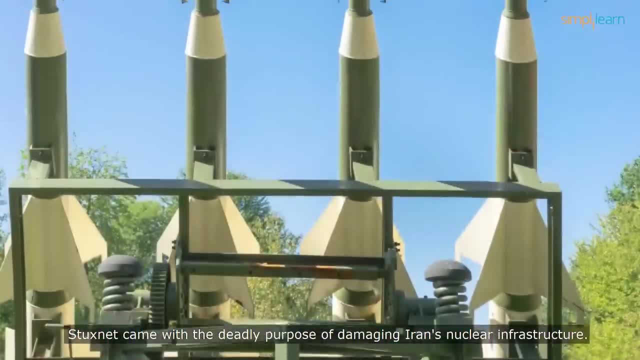 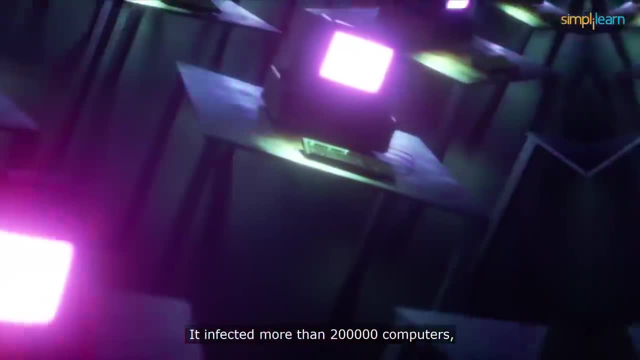 The project was actually planned by SAAG back in 2000, with the purpose of PinkCOOL, a transcontinental komputer company to discuss the future of mobile data and technology. From the very beginning, the project of the project was delusional. 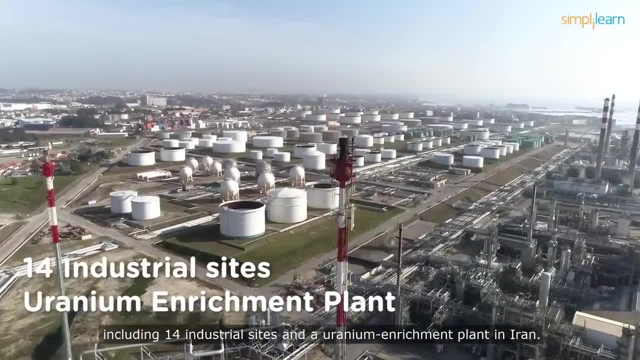 even though the title of the project was called the Digital S? prend and was included in theels of the project The first month it was released, a new version of the project was released In 2014,. it was the second month of the project. 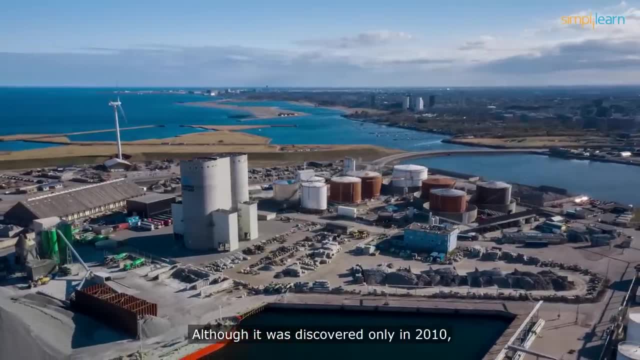 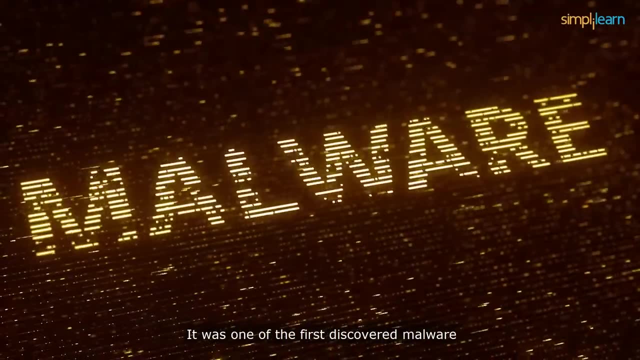 systems. Although it was discovered only in 2010,, it is believed to have been silently sabotaging Iran's nuclear facilities. It was one of the first discovered malware that was capable of hampering hardware systems. It largely damaged the centrifuges of the. 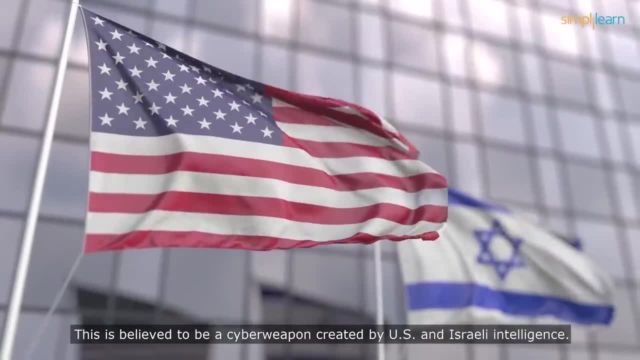 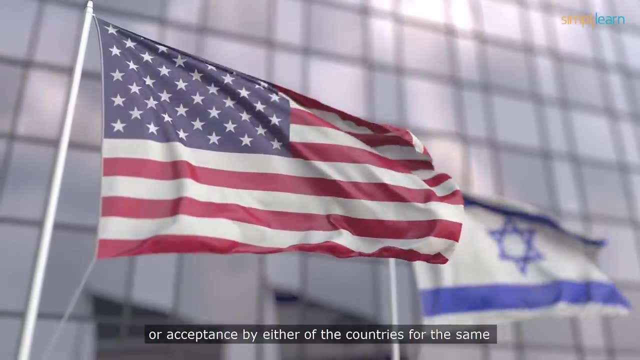 Iranian reactors. This is believed to be a cyber weapon created by the US and the Israeli intelligence, although there is no documented evidence or acceptance by either of the countries for the same. Moving on to number 4. In the year 2014,, Home Depot was the victim of one of the deadliest 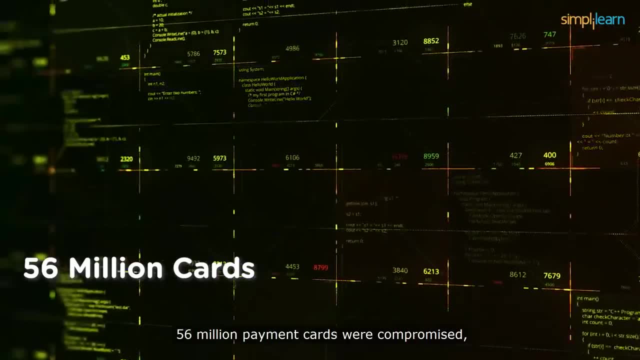 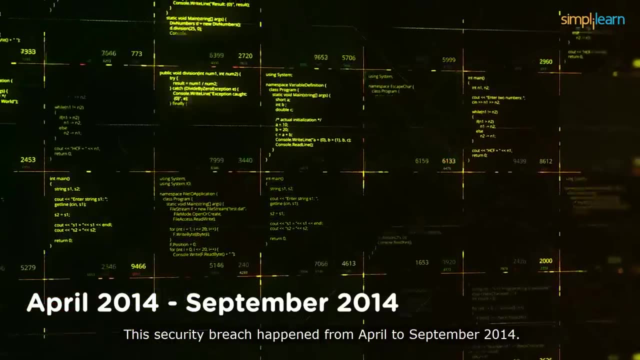 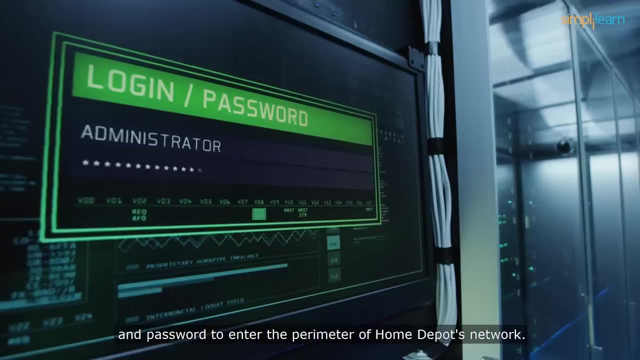 cyber attacks, 56 million payment cards were compromised, along with 53 million customer email addresses stolen. This security breach happened from April to September 2014.. Criminals were believed to have used a third-party vendor's username and password to enter the perimeter. 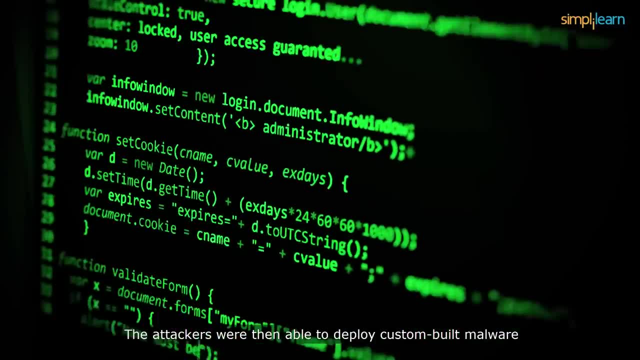 of Home Depot's network. The attackers were then able to deploy custom-built malware on its self-checkout system. The security breach happened in April 2014.. Criminals were believed to have used a third-party vendor's username and password to enter the perimeter of Home Depot's network. The attackers 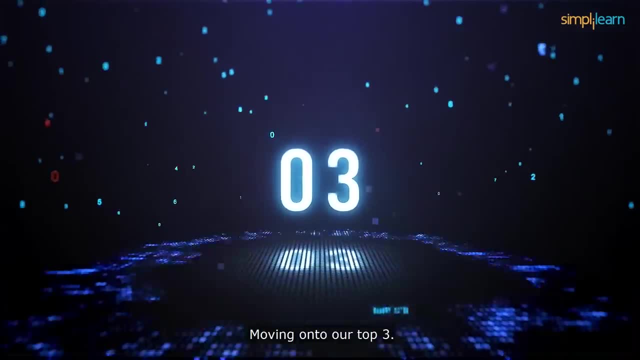 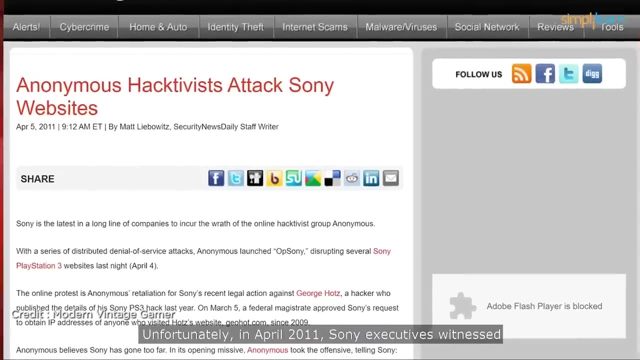 were believed to have used a third-party vendor's username and password to enter the perimeter of theıyorum. As you might be aware, the PlayStation gaming system is one of Sony's most popular products. Unfortunately, in April 2011,, Sony executives witnessed abnormal activity. 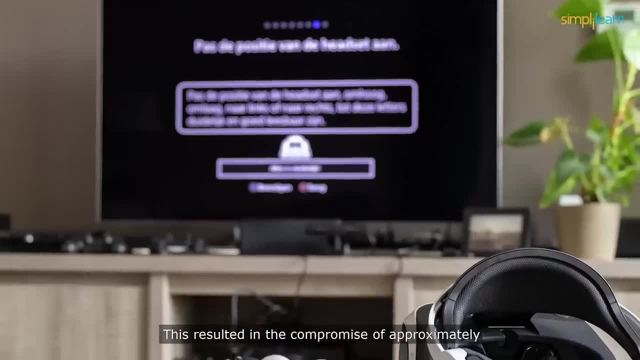 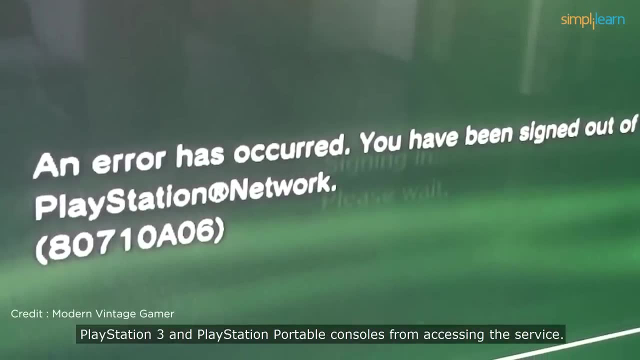 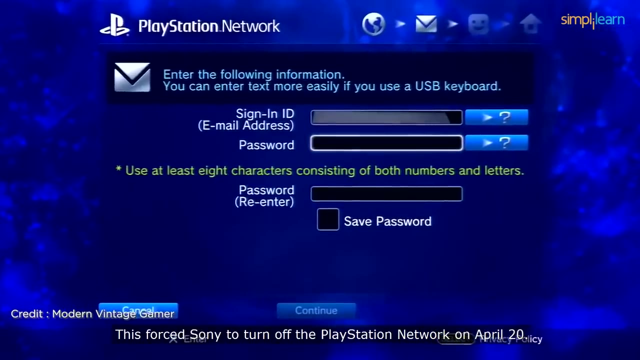 on the PlayStation Network. This resulted in the compromise of approximately 77 million PlayStation users' accounts and prevented users of PlayStation 3 and PlayStation Portable consoles from accessing the service. This forced Sony to leave the PlayStation Network. Sony to turn off the PlayStation Network on April 20.. 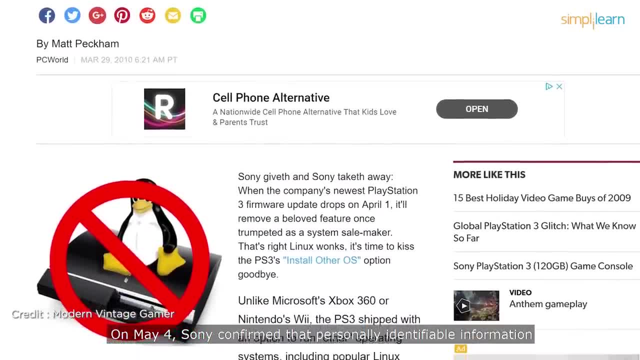 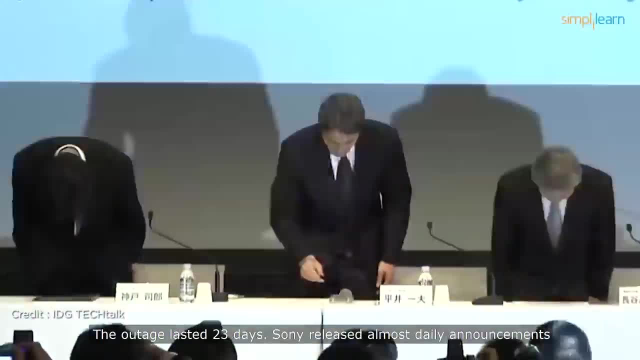 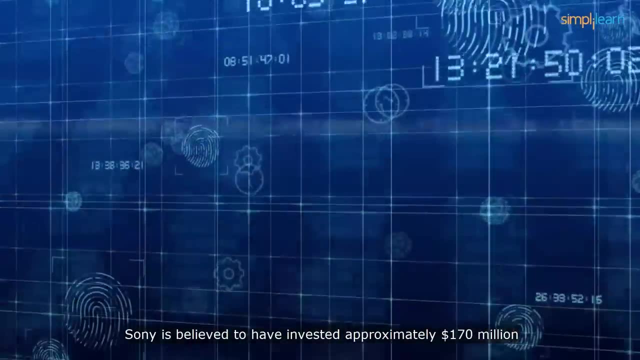 On May 4,, Sony confirmed that personally identifiable information from each of the 77 million accounts had been exposed. The outage lasted for 23 days. Sony released almost daily announcements concerning the system outage. In the end, Sony is believed to have invested approximately $170 million to improve the 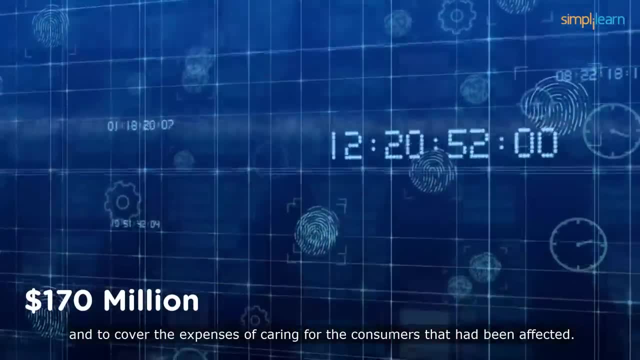 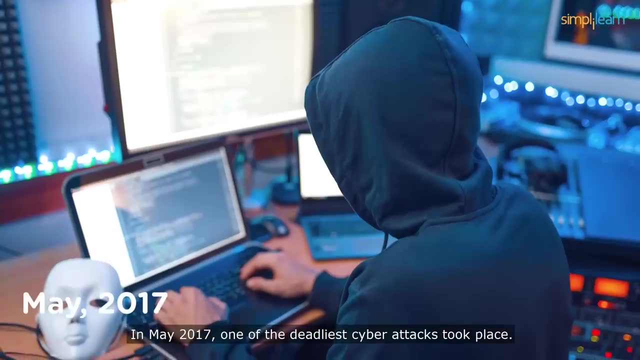 network's security, to investigate the attack and to cover the expenses of caring for the consumers that had been affected. Let's now move on to the next attack, at number 2.. In May 2017, one of the most dangerous cyberattacks took place. 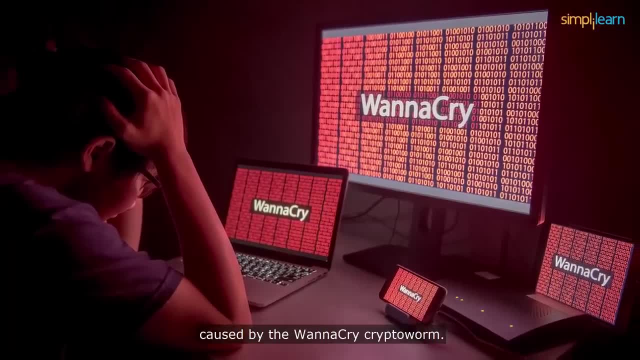 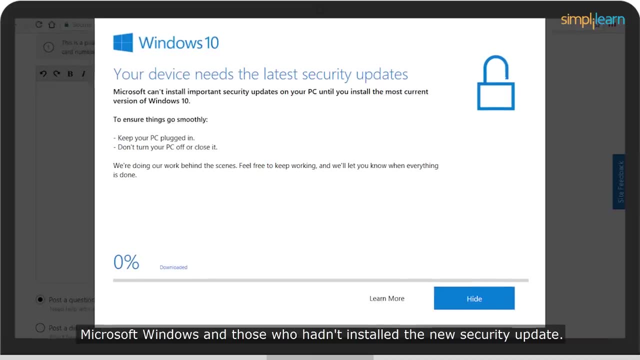 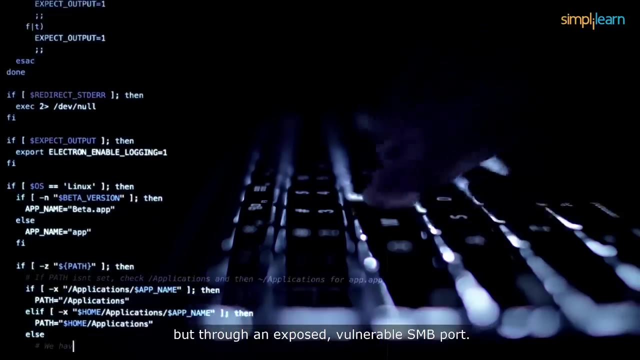 It was known as the WannaCry ransomware attack, caused by the WannaCry crypto worm. The victims were the users that used the unsupported version of Microsoft Windows and those who hadn't installed the new security update. This did not take place through phishing, like other attacks, but through an exposed vulnerable. 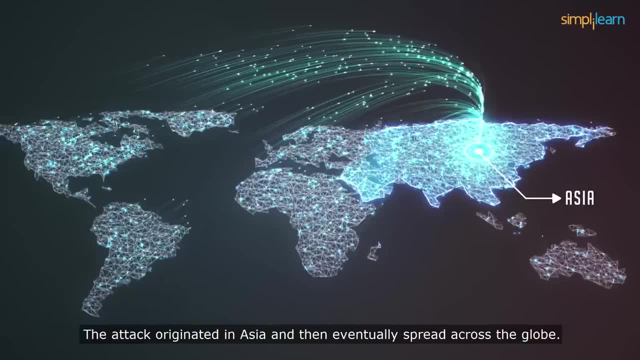 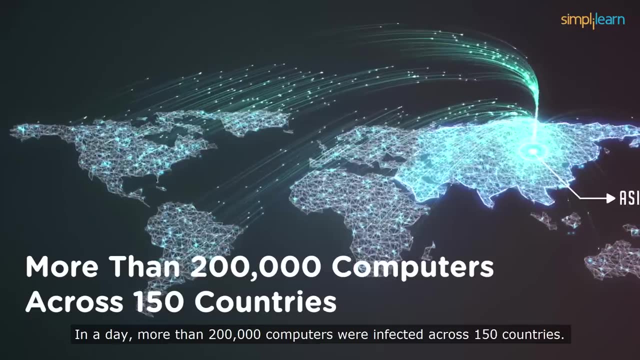 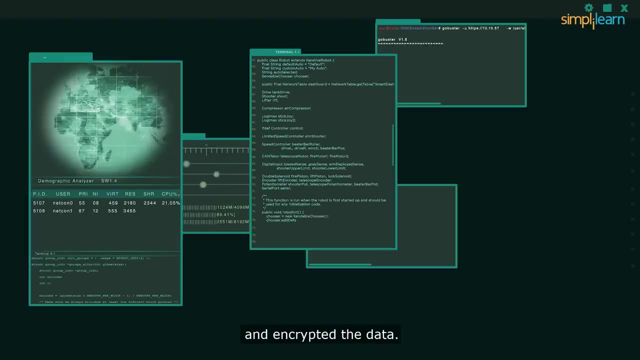 SMB port. The attack originated in Asia and then eventually spread across the globe. In a day, more than 200,000 computers were infected across 150 countries. The WannaCry crypto worm locked the users out of the targeted systems and encrypted their data. 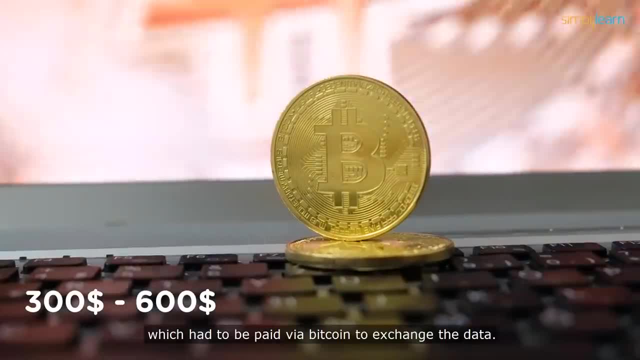 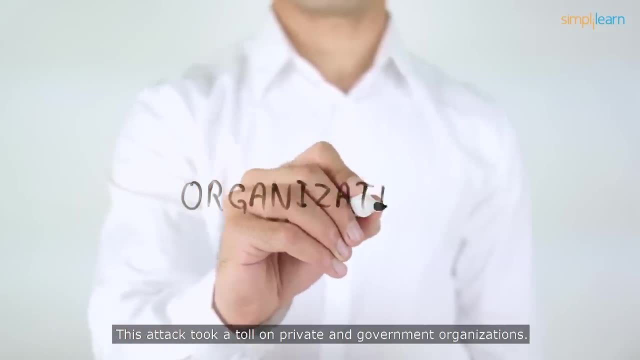 The users were asked for a ransom of $300 to $600, which had to be paid via Bitcoin, in exchange for their data. This attack took a toll on both private and government organizations. It resulted in damages from hundreds of thousands of people. The attack was the first of its kind. 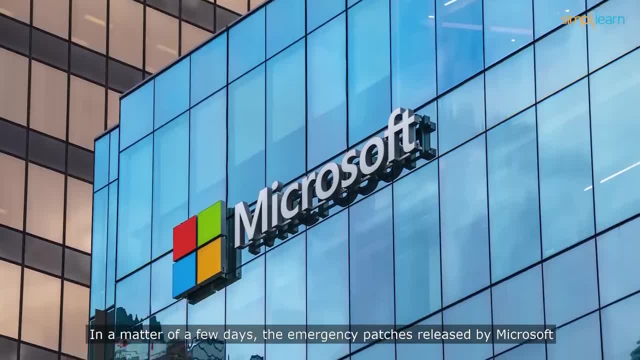 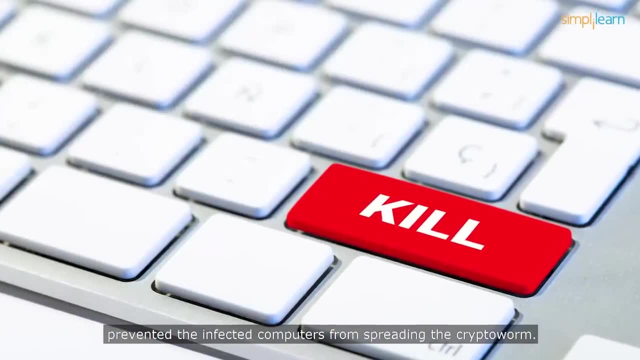 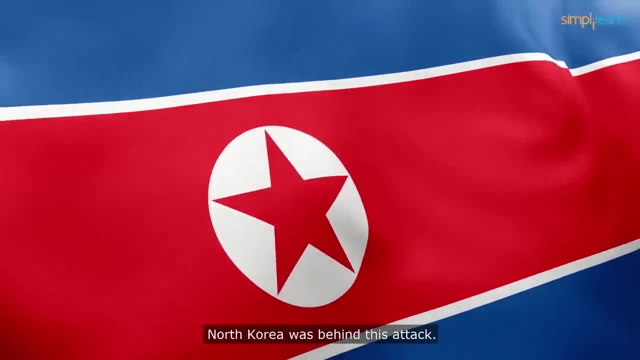 It cost millions to billions of dollars. In a matter of few days, the emergency patches released by Microsoft halted the attack. Also, the discovery of a kill switch prevented the infected computers from spreading the crypto worm. Security experts in a few countries believed that North Korea was behind this attack. 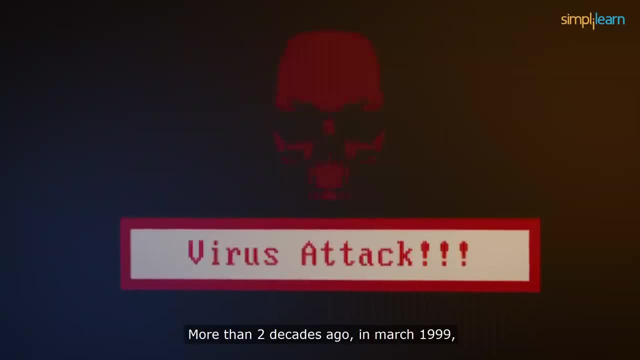 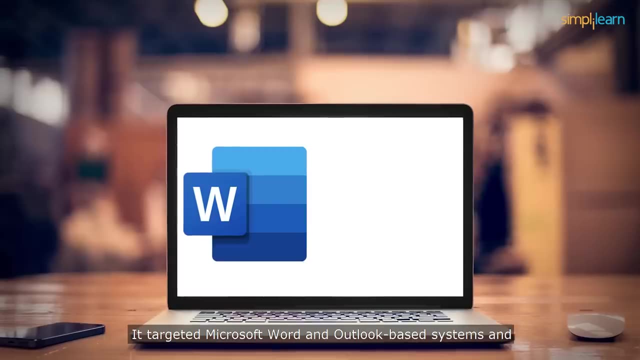 And finally, let's see what we have at number 1.. More than two decades ago, in March 1999, the Melissa virus, a mass-mailing macrovirus, was released. It targeted Microsoftcom. It used Microsoft Word and Outlook-based systems and created considerable network traffic.